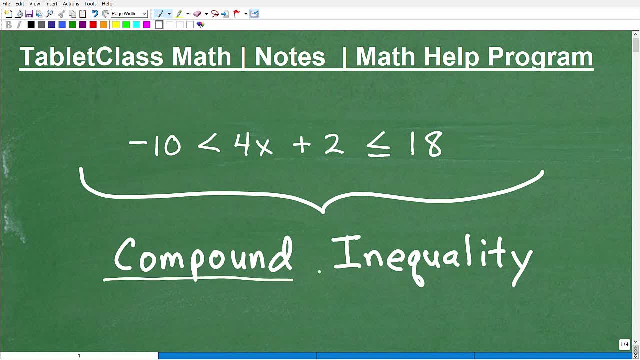 Okay, let's talk about compound inequalities. You can see here I have an example problem. I'm going to walk through how to solve this step by step. But if you're studying compound inequalities, this is a type of inequality and it's in contrast to another type called a linear inequality. 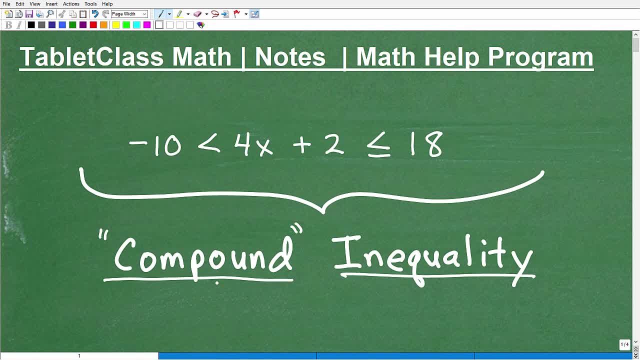 But with any inequality, you need to know how to graph the solution set to an inequality. So there's some other things that go along also with compound inequalities. the word and, and or come into play. So I'm going to quickly review these concepts as well, because obviously, if you're interested in compound inequalities, it's just more than just hey, how do you solve this problem real quick? 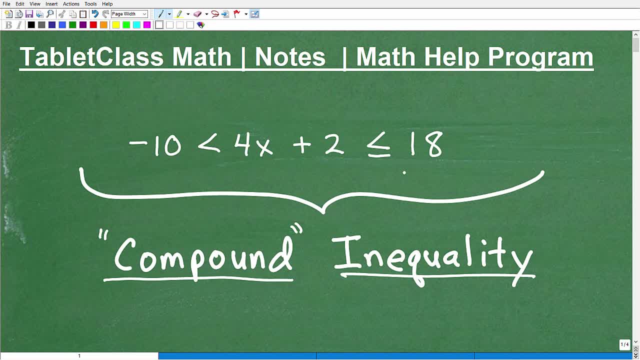 Okay, because if you're not quite sure and you're just solving this problem, chances are you might have questions about these other things. So as a math teacher, I am going to, you know, really help you out here. So I'm going to kind of try to keep this video. 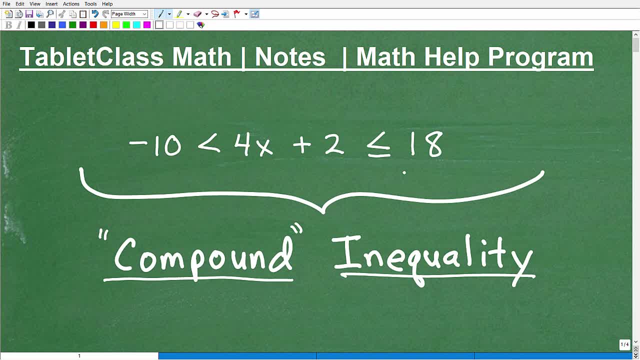 It's pretty short and direct, but we need to cover things that you we have to make sure you understand everything about inequalities. Okay, so I don't want you to walk away from this video without really having a quick review on all this stuff. 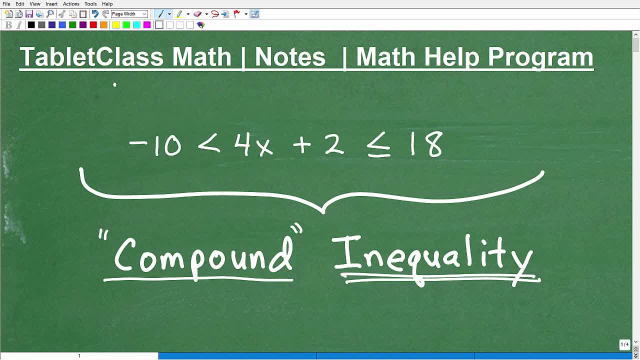 Okay, but before we get started, let me quickly introduce myself. My name is John. I'm the founder of Tablet Class Math. As I said, I'm also a middle and high school math teacher And over several years, I've constructed what I like to believe is one of the most powerful online video-based math help programs there is. 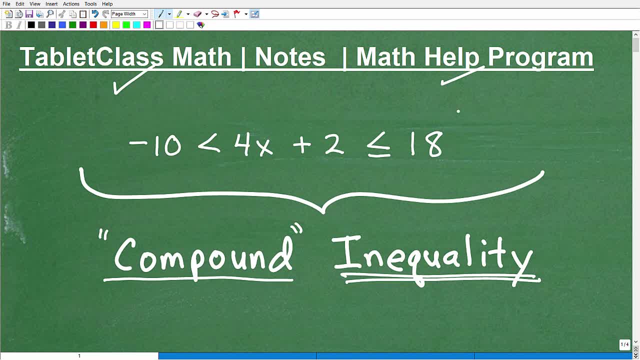 I'm going to link to that in the description. I'm going to leave a link to that program in the description of this video. So, whether you're taking a class or you need to take a full math class, my program can help you out. 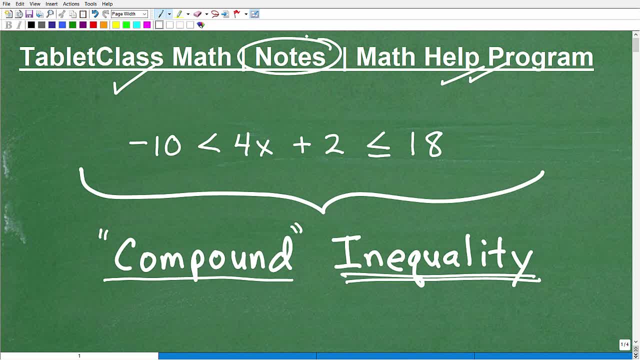 Now, as a math teacher, I just can't help to stress, every single time I speak to any math student, the importance of note-taking. Okay, how are your notes? If they're anything less than exceptional, then you're doing yourself a disservice in mathematics. 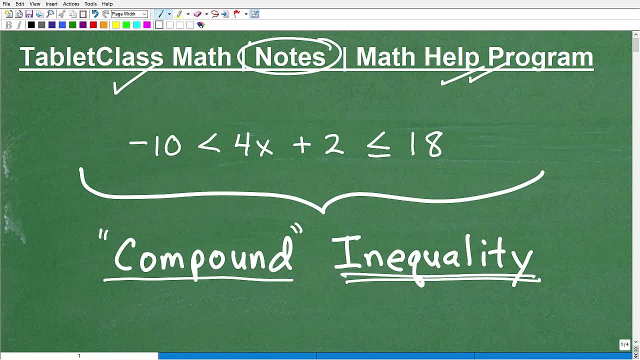 So, over decades of teaching math, there's one rule that I've seen, that I firmly believe- and I've just seen this over and over through the years- is those students with the greatest math scores in the world. they're the ones with the greatest math scores in the world. 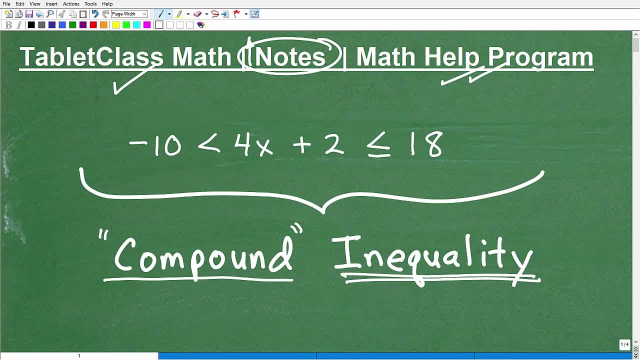 And those students with the greatest math notes typically have the greatest math grades. It's just a correlation that it's just a rule. I don't know if it's a rule of the universe, but it's a pretty solid rule. So if your math notes are not that organized or sloppy, or you don't take math notes, then you need to improve in this skill. 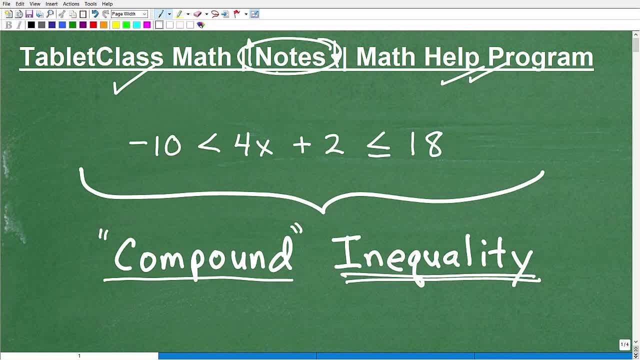 Don't take any shortcuts. You have to improve your note-taking if it's not absolutely excellent, But in the meantime you need something to study from. So I actually offer math. I'm going to leave a link to those very comprehensive, detailed math notes. 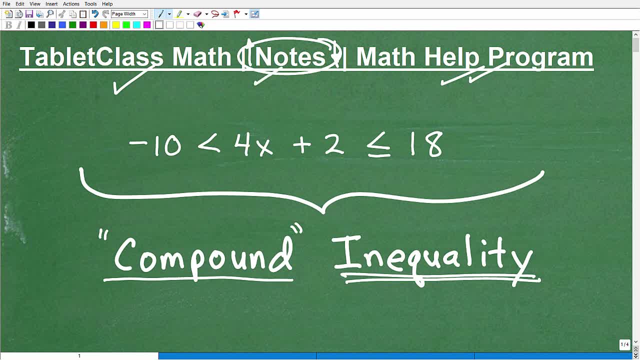 I'm going to leave a link to those in the description of this video as well. Those would include pre-algebra, algebra 1,, geometry, algebra 2, and trigonometry. All right, so let's get into this problem. 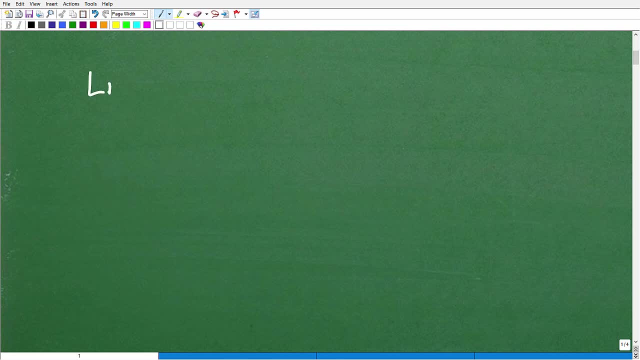 And so we're talking about compound inequalities. but let's just quickly distinguish compound inequalities versus another type of inequality, And that would be linear inequality. So a linear inequality would be something like 2.. So x is less than 8, or maybe x is greater than or equal to negative 9.. 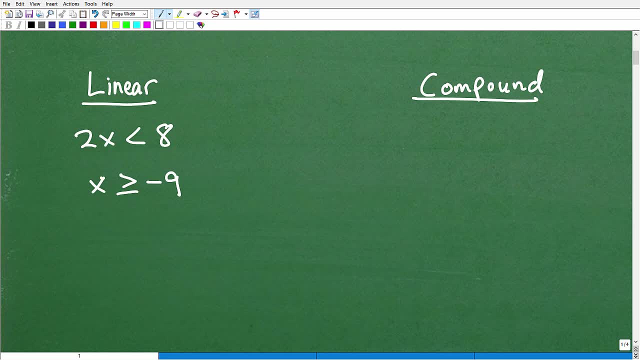 So there's just one situation here. okay, x is greater than or equal to a particular number, or less than or equal to a particular number. It doesn't make a difference. This is an example of a linear inequality, Now a compound inequality. there's more inequality symbols going on. 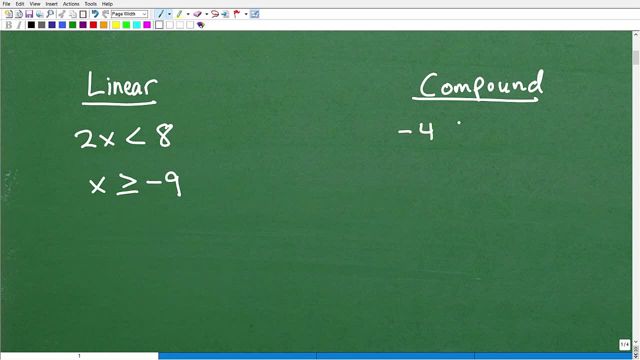 So, for example, negative 4.. Well, x would be greater than negative 4, but at the same time less than or equal to, let's say, 10.. Okay, this is an example of a compound inequality, because we're stating two things here. all right, 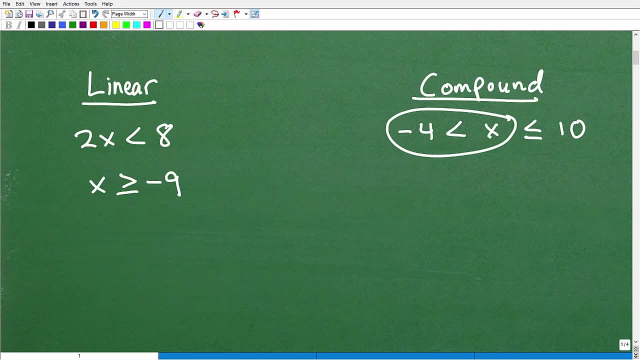 So we have. it's almost like you have two linear inequalities going on. You have hey x. this number is greater than negative 4, but at the same time it's got to be less than or equal to 10.. 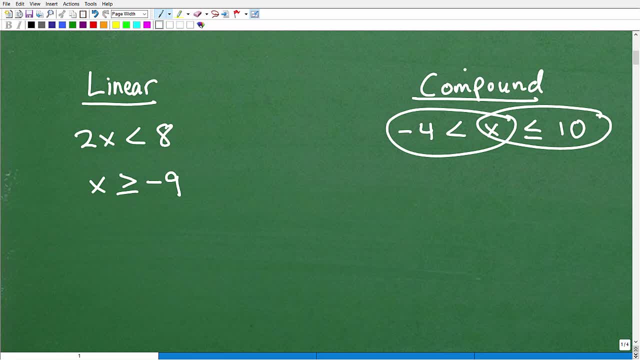 So that's the idea between compound. Compound kind of implies two things, right, So this is a range of values. So we're talking about compound inequalities, If you just looked at this problem here I'm saying in this number, okay, numbers, x, right represent numbers. 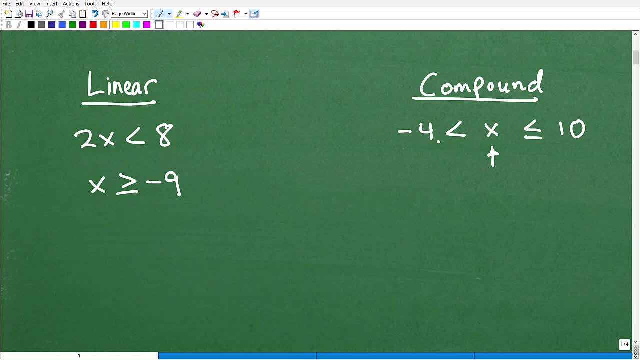 I'm saying, have to meet two conditions: It has to be greater than negative 4- and okay, I'm using this word- and at the same time, less than or equal to 10.. So this and all right implies a graph that looks like this: all right. 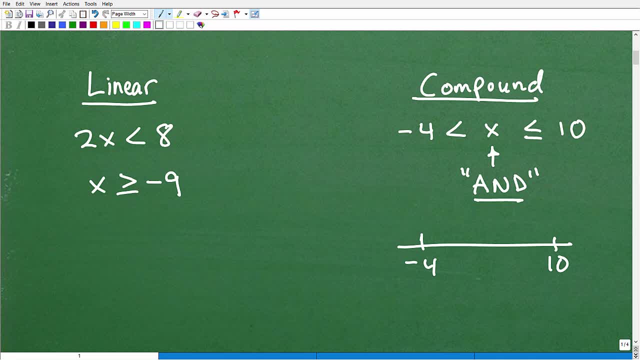 So if you're not familiar with graphing inequalities, then kind of have to go back and review linear inequalities. but we'll touch on that here. Okay, so the graph would be like this: We're going to fill in this circle at 10, okay. 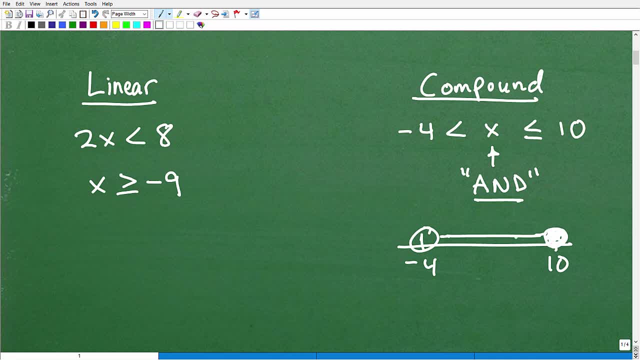 So all these numbers, not including negative 4, all this range right here to include 10 would be the solution set. Now. this is an and statement: all right, X, give me all x's that are greater than negative 4.. 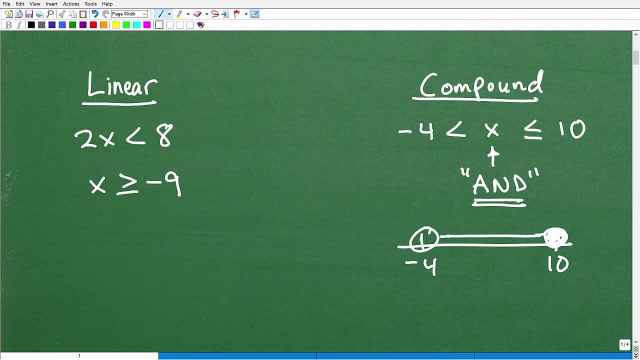 And, at the same time, less than or equal to 10, okay and all right. So that's what we're talking about, But I kind of like to think of when we're talking about the graphs, so you don't confuse this. I like to think of the word hand, all right. 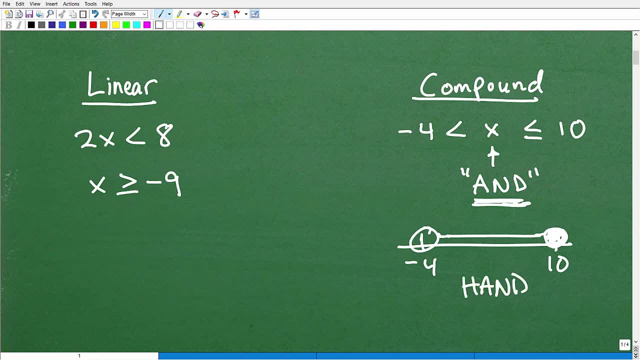 So, and you think of the word hand. all right, Now, why would I say that word? Well, this kind of looks like a handlebar on a bike, okay, So here's maybe a little bike in here. Here's the tire of the bike and the pedals, right. 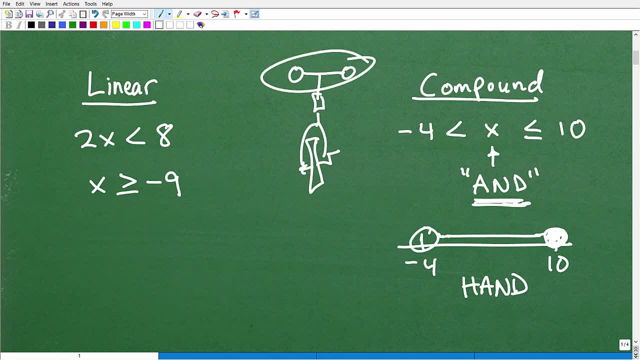 So here, when you're thinking and you're like: oh, the graph is going to be like a bar, like a handlebar, okay, Now that would be in contrast to- let me go ahead and erase this guy over here- the word or right. 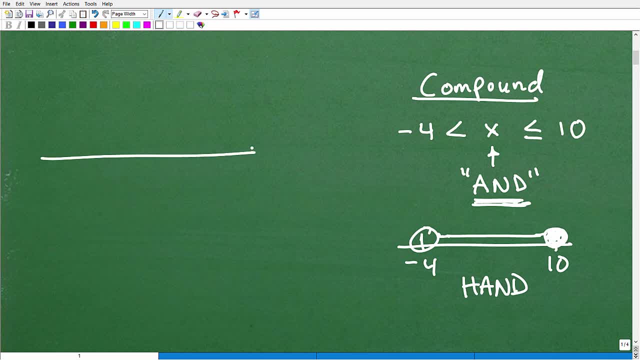 So what would that look like? Well, the graph would look like this: Let's see if we can reconstruct the actual compound inequality. but it would be something like this: Let's use the same numbers, 10 and negative 4.. Okay, so something like this: 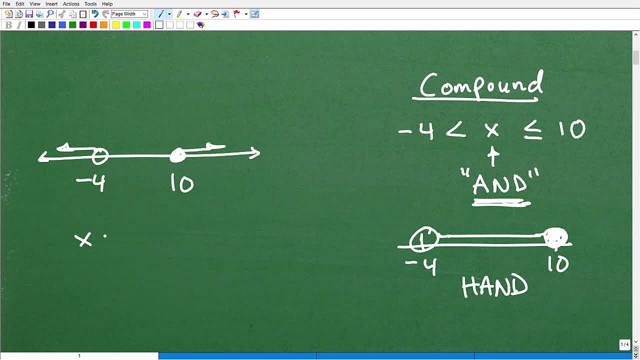 So what am I saying here? I'm saying all x's. give me all x's that are less than negative 4 or okay, or greater than or equal to 10,, okay. So this is another example of a compound inequality. 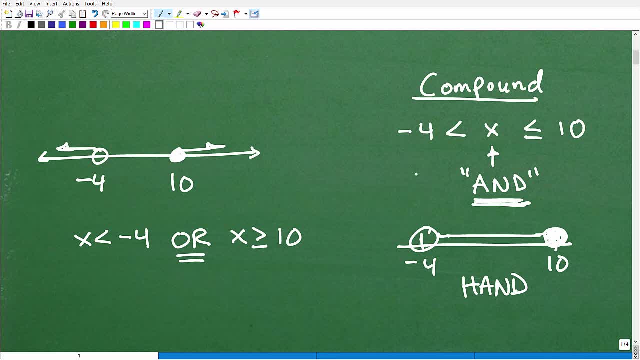 Now, sometimes, when you're, you can have an inequality that kind of looks like this, and when you solve it, you can end up with an or statement. all right, So an or statement. the solution set is these numbers, Okay. 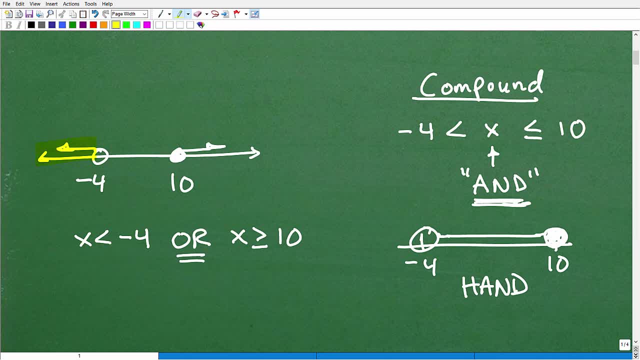 So all numbers over here, okay, all numbers that are less than negative 4 or okay, numbers that are greater than or equal to 10, okay. So these are the solution sets and we represent solution sets by graphs for compound inequalities and linear inequalities as well. 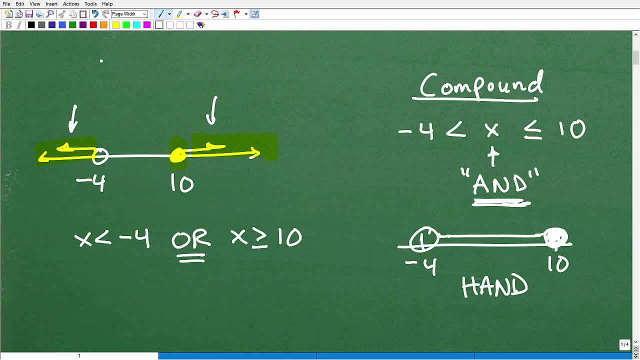 So now look at this or graph. okay, It looks like this, okay, Like kind of like that. Now I like to think of that as like the ors on a little boat, Like here's a little rowboat. 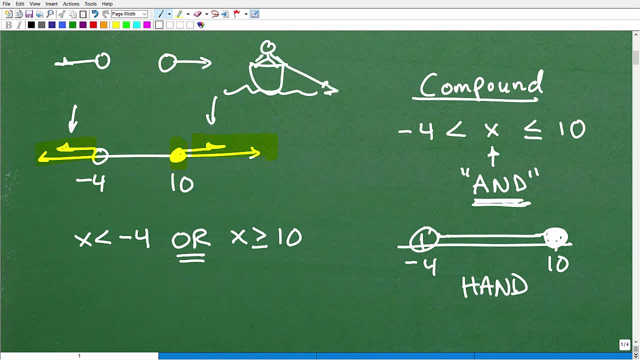 Here's a person, Here's a person in the boat, and they got their little ors out like so, okay. So the graphs going this way, okay, are going to be the graphs of an or statement versus our and statement, which is going to be like handlebars. 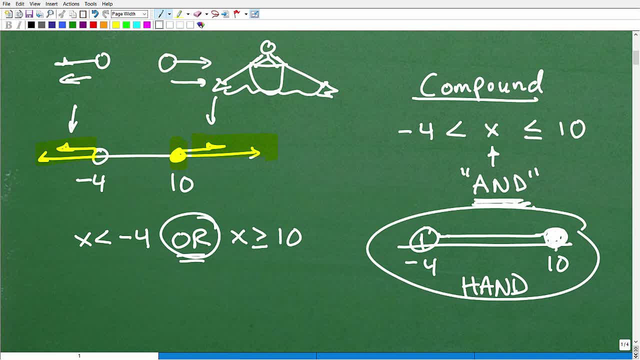 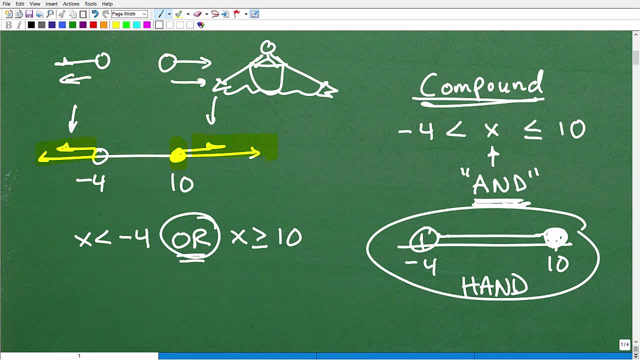 you're going to have to, you know, also really be have a firm grasp on these words and and or and their respective graphs. Okay, let's get into this problem now, And once you understand this, then this is fairly easy stuff. 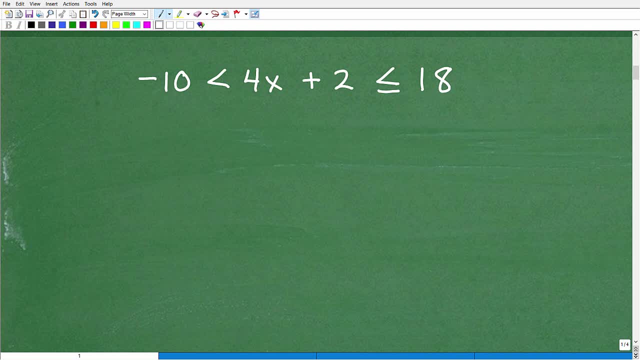 All right, so here's our inequality. okay, The one thing I want you to know is that the way we solve a compound inequality is pretty much we're taking the same steps as if we're solving an equation, But effectively what we're going to do is kind of solve for x. 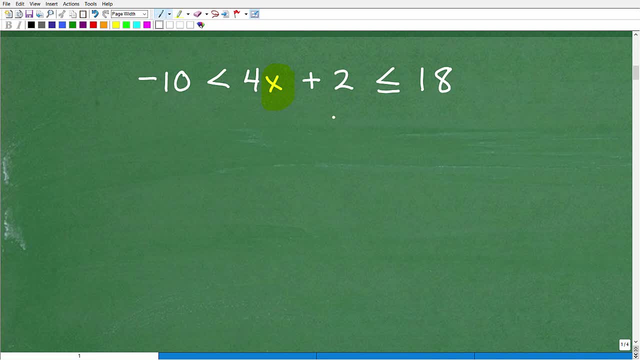 And we're going to take x in the middle, okay, So if this was an equation, what would I do? I would subtract two from both sides of the equation, But here I need to subtract two from all sides of the inequality. 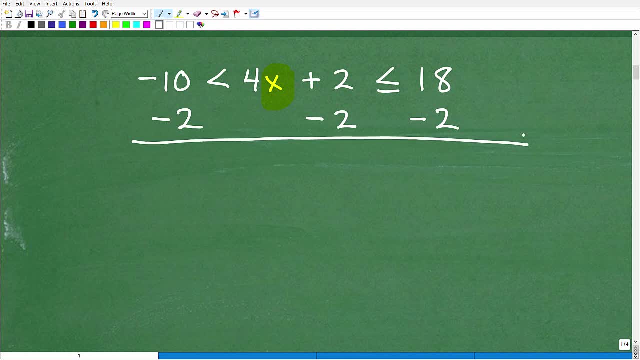 So it would look like so. okay, So that's going to be our first step. So when we add down, I'm going to get negative 12,. all right is less than I got my 4x in the middle here, less than or equal to positive 16.. 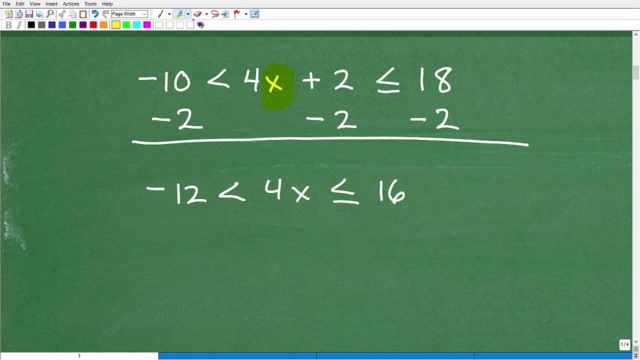 Okay, So I'm going to do this Pretty straightforward, but again, what I'm trying to do is to get x by itself. So how can I do that? Well, I'm going to divide everything by 4,, all right. 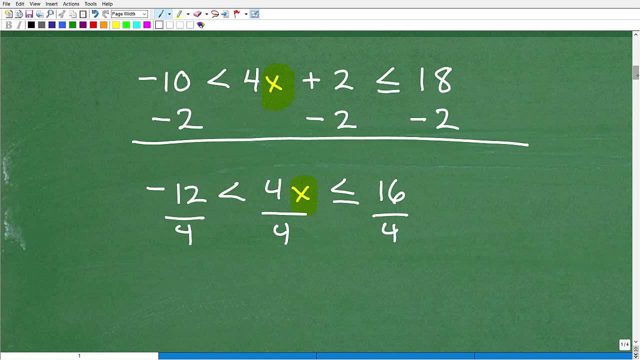 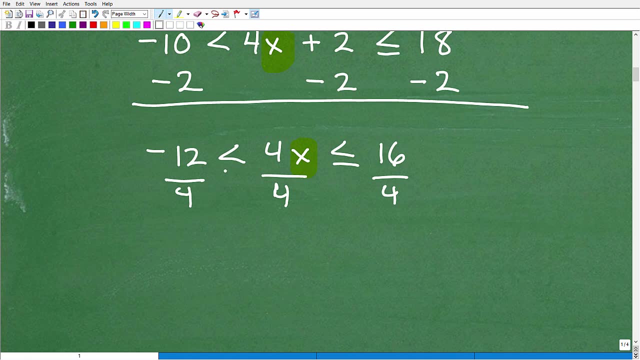 Now here's the thing: okay, If that was a negative 4, okay. Remember, when you're dividing it by a negative number, when you're working with inequalities and you divide by a negative number or multiply by a negative number, your inequality signs will reverse. 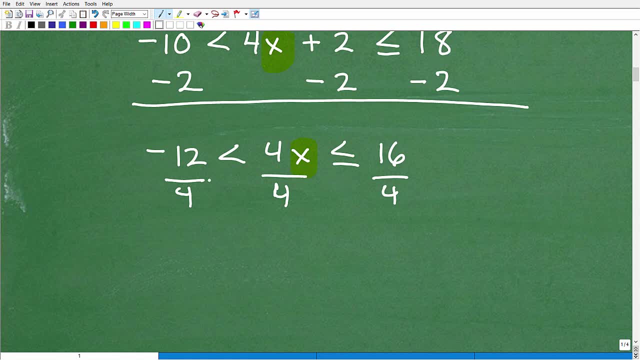 Here this is a positive number, so nothing's going to reverse. So let's go ahead and simplify. So negative 12 divided by 4 is negative 3, and that's going to be less than x. And then here I'm going to have less than or equal to a positive 4.. 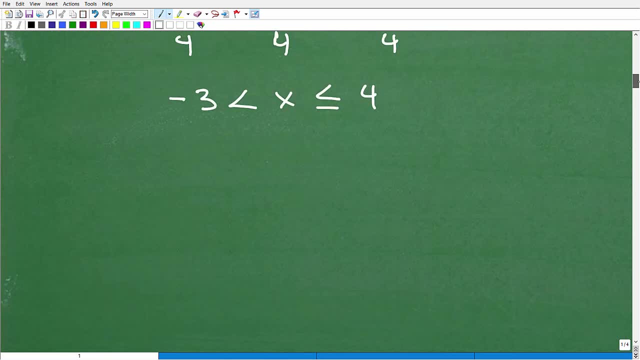 Okay. so what kind of statement is this? Is this an and or an or? Okay, and how can we graph this? Well, we're saying: give me all x's that are greater than negative 3 and, at the same time, less than or equal to positive 4.. 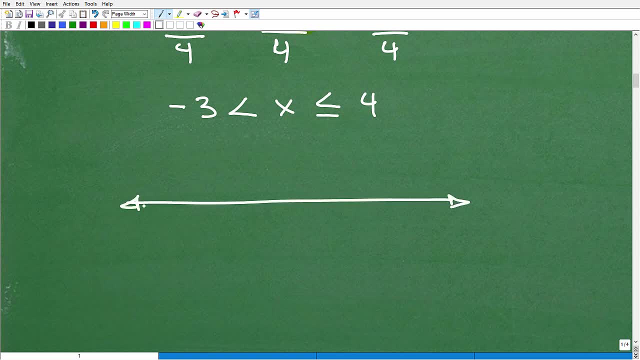 So I can just go ahead and graph that real quick. The easiest way to do that is just to plot these two numbers, put two circles like so: okay, Now I know that this is an and statement, so it's going to be a handlebar type of graph. 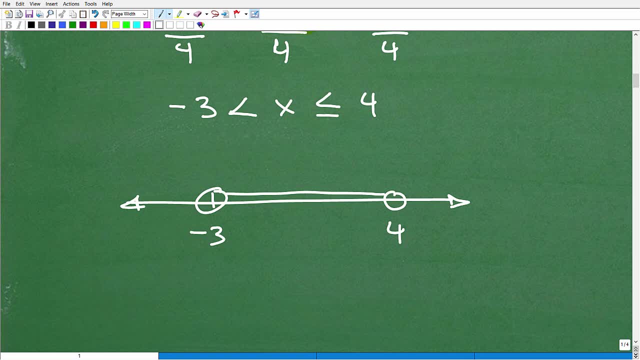 So an open circle is only for greater than: okay, I don't have an equal to, so I'm going to leave that open. And then that positive 4, I've got to fill that in. So this graph is saying all numbers that are greater than negative 3.. 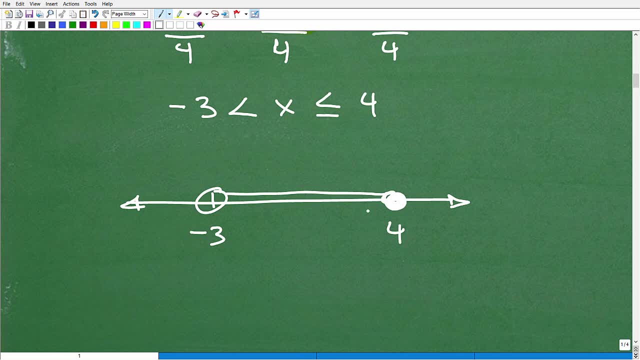 Negative 3, 2, positive 4, up and to include positive 4, and this would be the graph. So this is the solution and this is the graph of that solution, And oftentimes you'll be given a graph and you'll need to kind of reconstruct that. 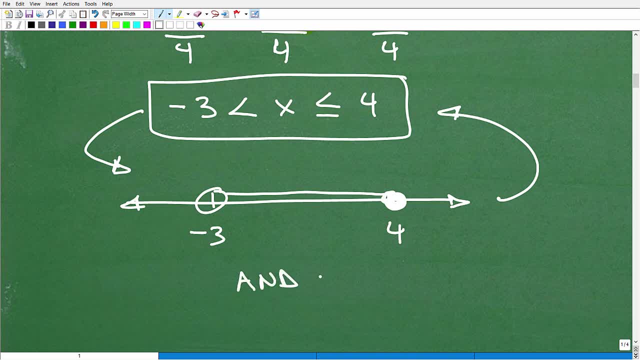 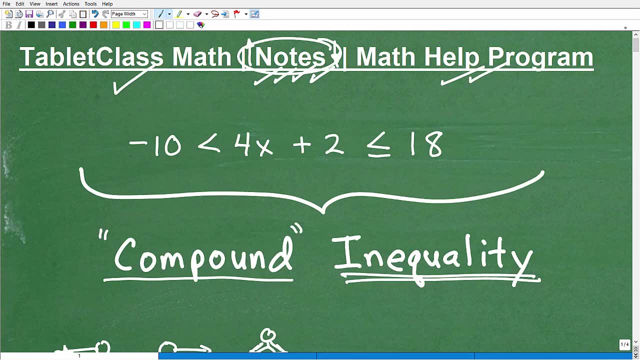 But the main thing, too, is to really understand the difference between and and or statements when we're talking about compound inequalities. All right, so let's go ahead and wrap up this video, Now that you're a complete expert on compound inequalities.